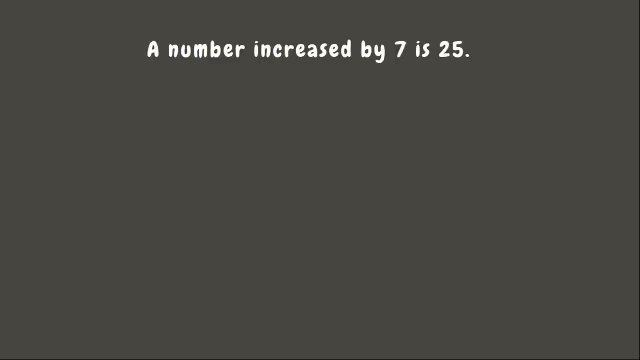 We have here a number: Increase by 7 is 25.. First we need to translate this one into one equation. We have a number which is missing or unknown, So let us represent this by a variable. Let m be our variable. 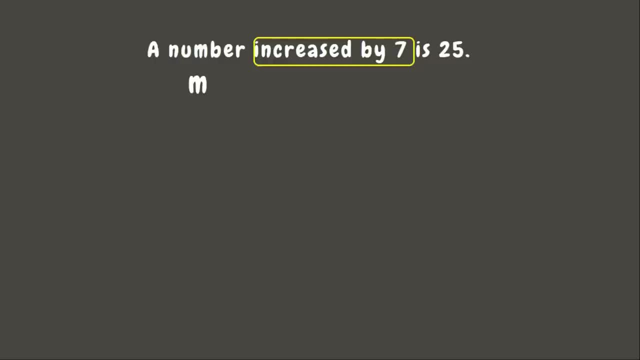 Next one: we have increase by 7,, which means addition, So that is plus 7.. And lastly, we have is 25,, which means equals 25.. Now our equation is m, So we have m plus 7, equals 25.. 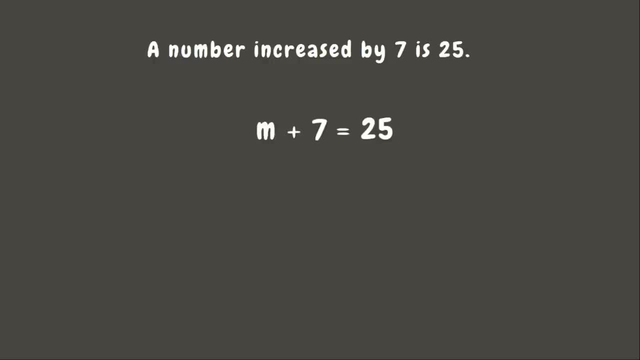 Now, solving for equations means finding the value of the variable. To solve for the value of the variable, we need to separate or leave it alone in one side. This means that we need to get rid of the constant 7.. But how are we going to do that? 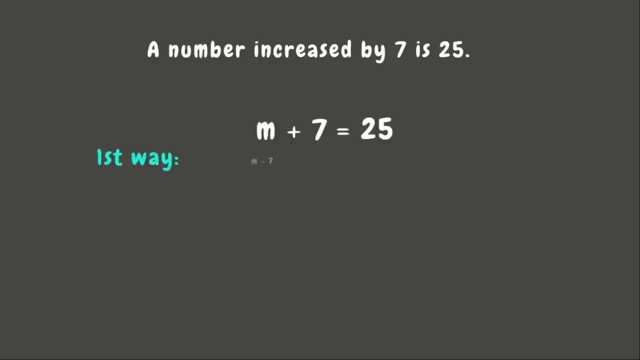 Let's see our first way To get rid of our constant plus 7,. we need to get its opposite operation, which is subtraction. Therefore, we are going to subtract 7 here. There you go Now. always remember that whatever we do in one side, we also need to do it on the other side. 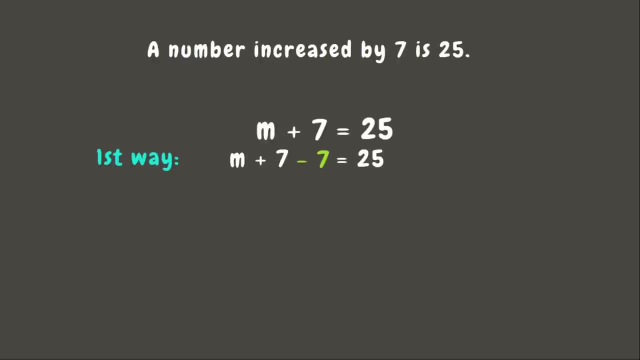 Since we subtract 7 on our left side, we are going to subtract 7 on our right side. There, Now it's time to solve. So here we have 7 minus 7, which is 0. So we can simply cancel this out. 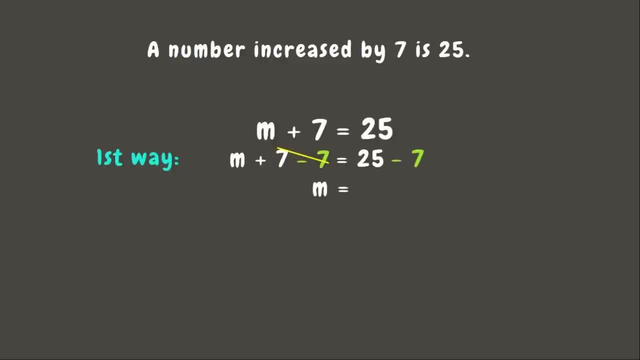 That leaves us the variable f. On the other side, we have 25 minus 7,, which is 18.. Great job. Therefore, the value of our variable is 18.. Now let's try to answer this one using our second way. 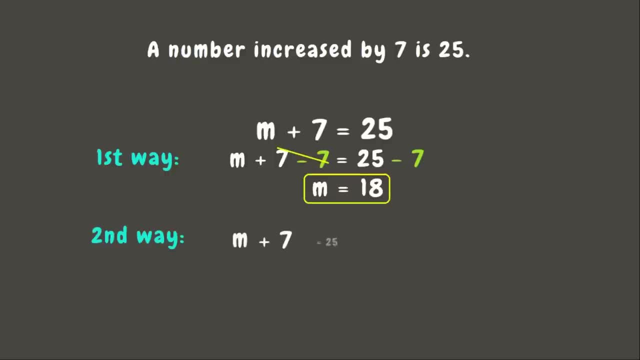 Again, our equation is: m plus 7 equals 25.. And for our second way, we are going to get the opposite operation of our constant. Since we have plus 7, the opposite is 0. The opposite is minus 7.. 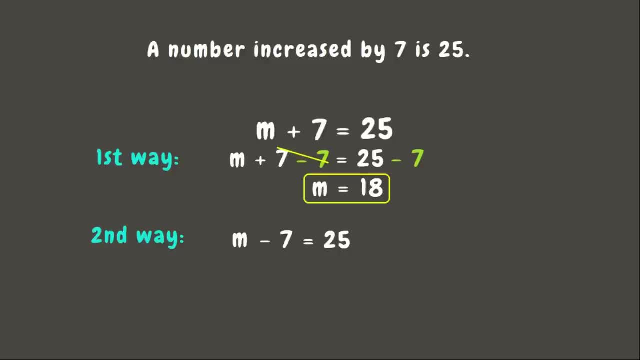 And the next thing that you are going to do is to move it on the other side of our equation. There you go. Now we have m equals 25 minus 7.. Now let us solve: 25 minus 7 is Great job, It's 18.. 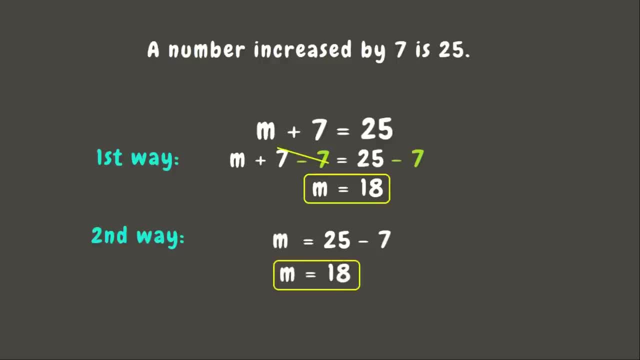 And we got the same answer. Now for us to make sure if our answer is correct, let us check. To check. if our answer is correct, we need to substitute the value of the variable that we got into our equation There. Now our answer is correct. 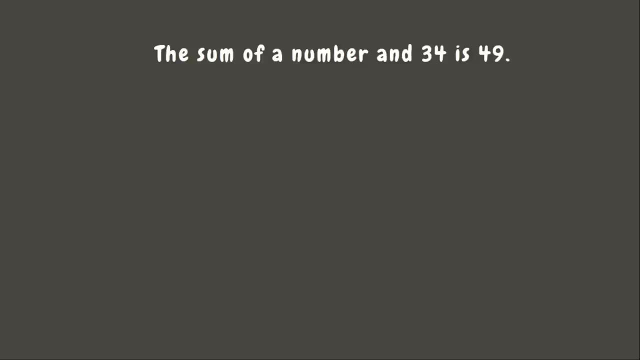 Let's go and have another example. This time we have the sum of a number, and 34 is 49. So let us translate this one first into one equation. We have the sum of a number and 34.. The sum means addition. 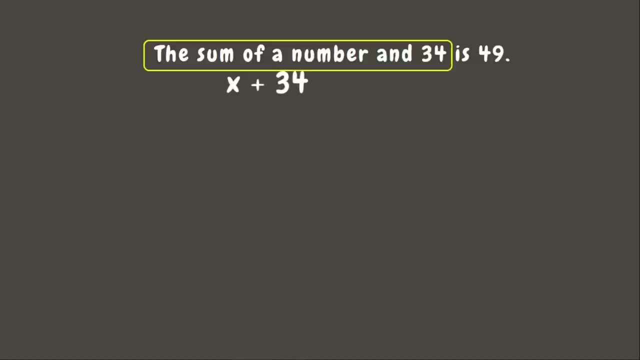 So that is x plus 34.. Which is 49. So that is equals 49. Our equation is: x plus 34 equals 49. Again, we need to remember that to solve for the variable we need to separate or leave it alone in one side. 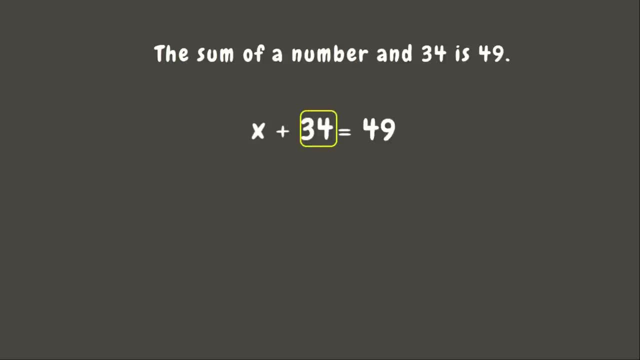 Therefore, we need to get rid of our constant 34.. Now, since it is addition, we need to get its opposite, which is subtraction. Therefore, we need to subtract 34.. And again, we need to remember that whatever we do on one side, we also need to do it on the other side. 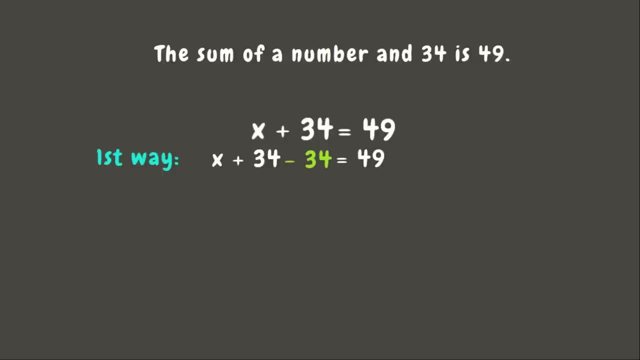 So, since we subtract 34 on our left side, we are also going to subtract 34 on our right side. There you go. Now let us solve. So we have here 34 minus 34, which is 0. So we can simply cancel this out. 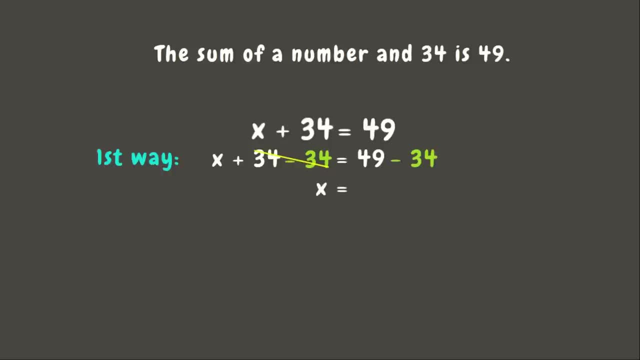 And that leaves us the variable x. On the other side we have 49 minus 34.. And that is wonderful, It is 15.. Now let us try our second way. Again, our equation is: x plus 34 equals 49.. 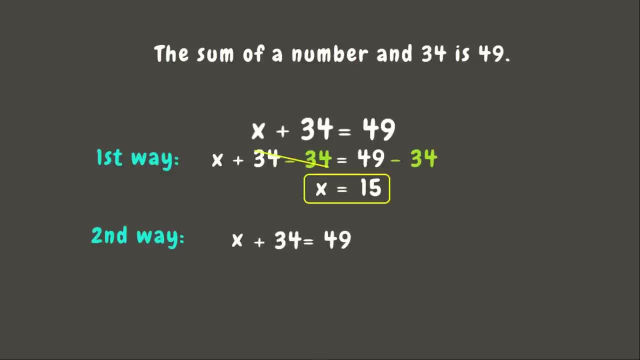 So the first thing that you need to do is to get the opposite of our constant Plus 34. Which is minus 34. And then move it into the other side of the equation, So that gives us x equals 49 minus 34.. 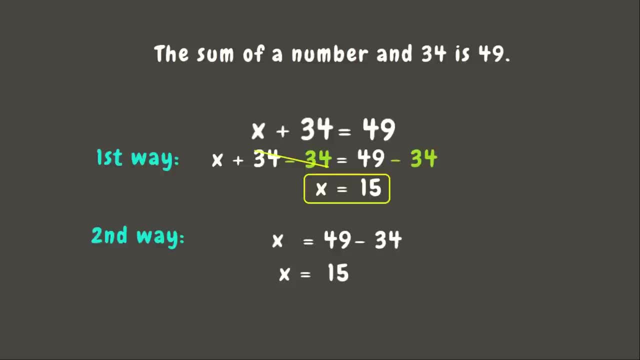 49 minus 34 is 15.. Wonderful, We just got the same answer. Now, to check for our answer, let us substitute the value of the variable. Now, our answer is correct. Now let us move on to our next example. This time we have 6 less than a number is 24.. 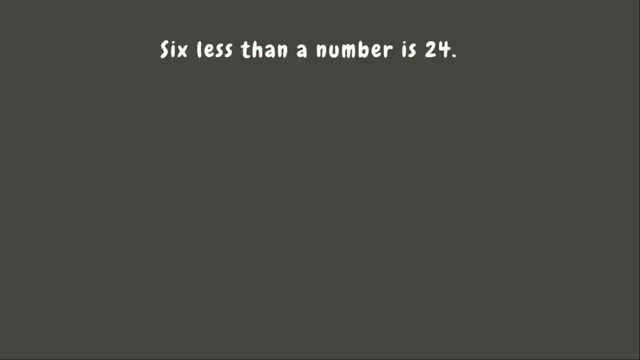 Again, let us translate this into an equation. So first we have here 6 less than, which means subtraction, So that is minus 6.. And next one we have a number, which means missing, So we can represent this by a variable, Let us say variable y. 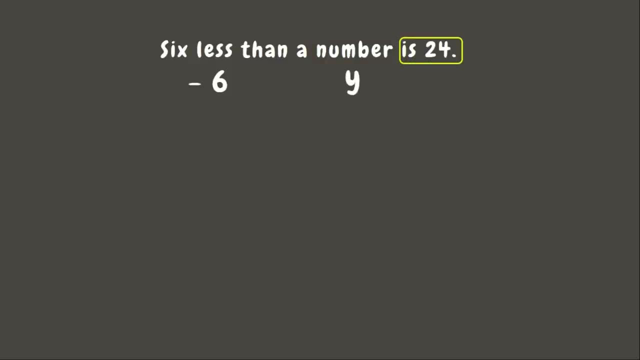 And next one we have is 24, which is equals 24.. Now let us solve Again. we need to get rid of our constant, to leave the variable alone in one side. So for our first way, we have y minus 6.. 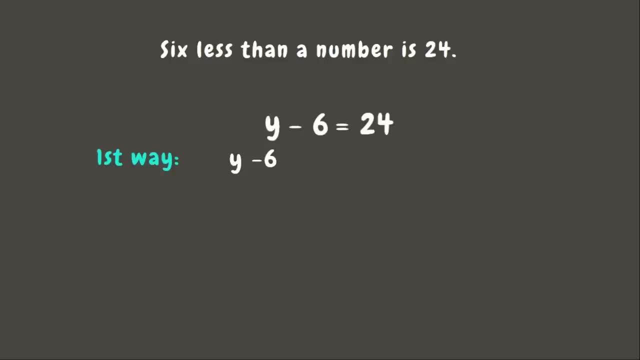 The opposite operation of minus 6 is plus 6.. Therefore, we are going to add 6 here, And since we add 6 on the left side, we are going to add 6 also on the right side. There you go. 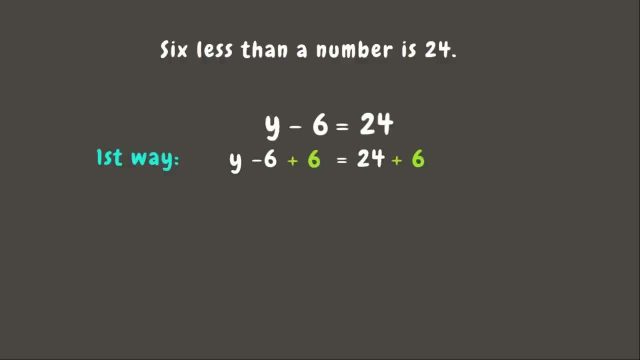 Now we can see here we have negative 6 plus 24.. And that is 0.. So we can simply cancel this out, And that leaves us our variable. y equals 24 plus 6, which is 30. Great job. Therefore, the value of our variable is 30.. 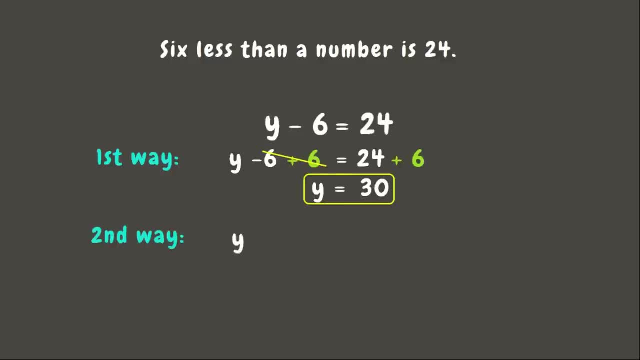 Now let us try using our second way. First thing that we need to do again is to get the opposite of our constant, which is negative, 6 or minus 6.. And the opposite of this one is plus 6.. And the next thing that we are going to do is to move this one into the other side of the equation. 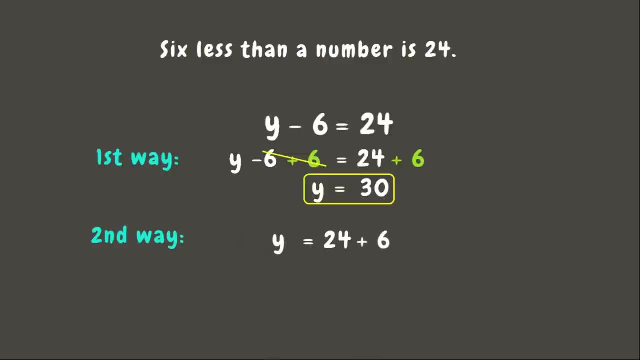 There We have 24 plus 6 is 30. Great job, Now let us check our answer. There you go. Now let us have another example. This time we have the difference of a number, and 9 is 60. Again, let us translate this one first into an equation. 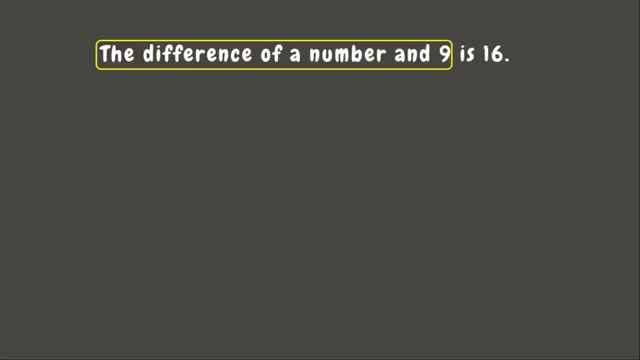 The difference of a number and 9.. So this means subtraction. So we have: x minus 9 is 16, which is equals 16.. Now let us solve for the variable by getting rid of the constant. Now let us try our first way. 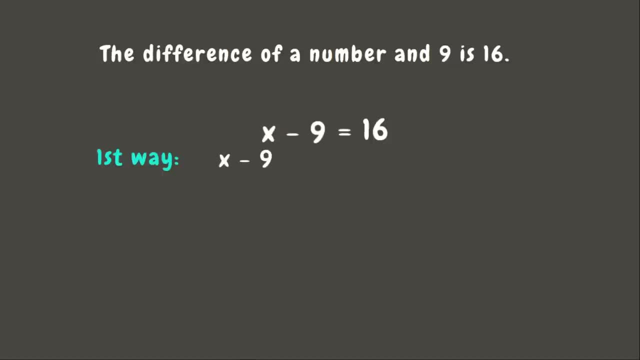 So we have x minus 9.. Again, we need to get the opposite of minus 9, which is plus 9.. Then we need to do it on the other side too. There Now let us solve. So we have negative 9 plus 9, which is 0.. 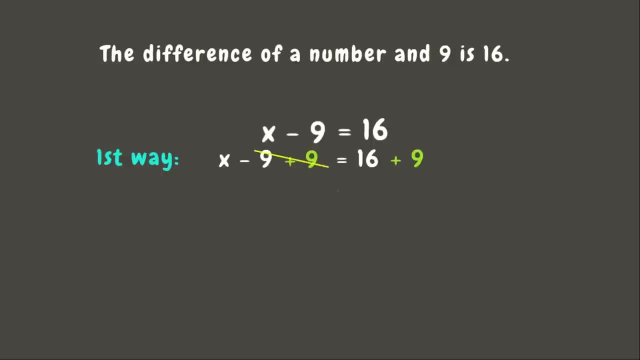 So let us cancel this out. And that leaves us the variable x, Next one. on the other side, we have 16 plus 9. And that is 25.. Very good, Now for our second way. we have again our equation: x minus 9 equals 16.. 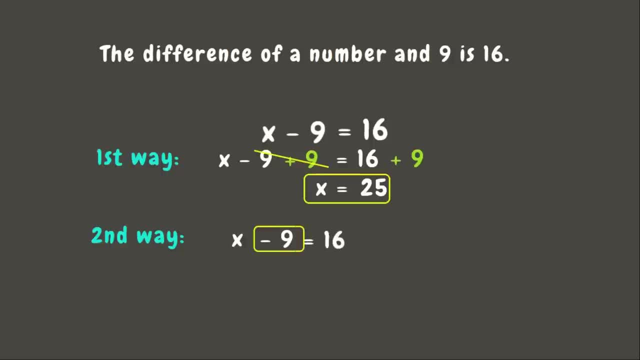 So again, we need to get the opposite of minus 9, which is plus 9.. And move it on the other side of the equation There. So we have x equals 16 plus 9, which is 25.. Great job. Now let us check our answer. 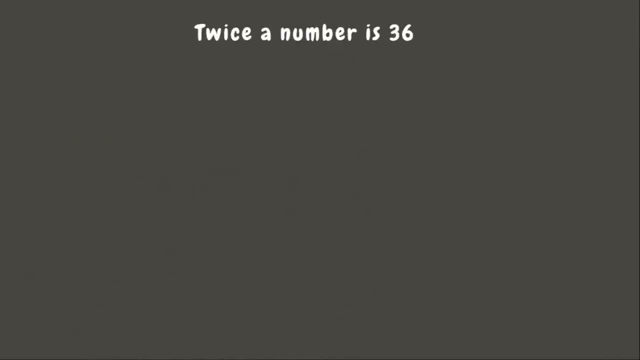 Awesome. Now let us have another example. We have twice the number is 36.. So let us translate this one first into one equation. So we have twice the number, which means 2 times a number, So that is 2 times b or 2b. 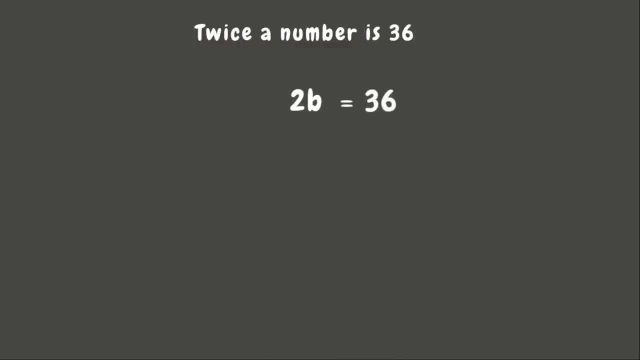 Which is equals 36.. So again, to get the value of the variable, we need to separate or leave it alone on one side. Therefore we need to get rid of the coefficient 2.. But how are we going to do that? Let's have our first way. 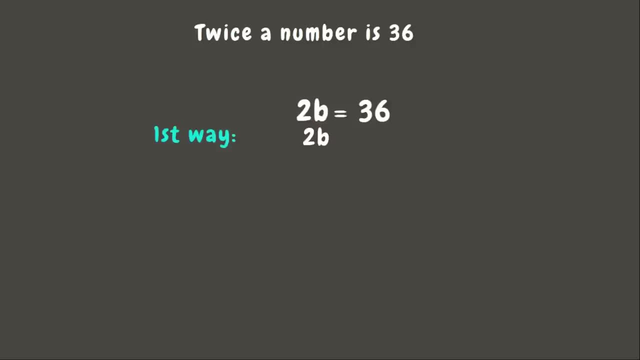 So, like we did earlier, We can get rid of the coefficient 2.. We can get rid of our coefficient or our constant value by getting its opposite operation. So, since this is multiplication, which is 2 times b, We can get rid of the coefficient 2 by division. 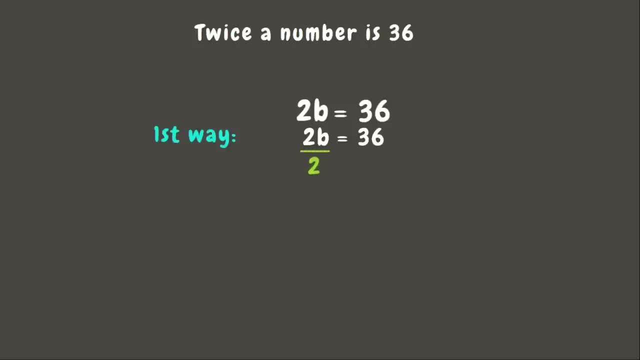 So we need to divide 2 on both sides. Now we have 2b divided by 2 equals 36 divided by 2.. Now to cancel out the coefficient, that is 2 divided by 2, which is 1.. So we can simply cancel this out. 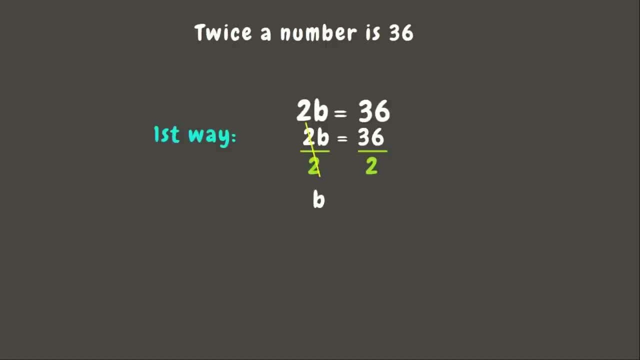 And that leaves us the variable b, While on the other side we have 36 divided by 2, which is 18.. Great job. Now let's have our second way. Again, our equation is: 2b equals 36.. Now to get rid of the coefficient 2.. 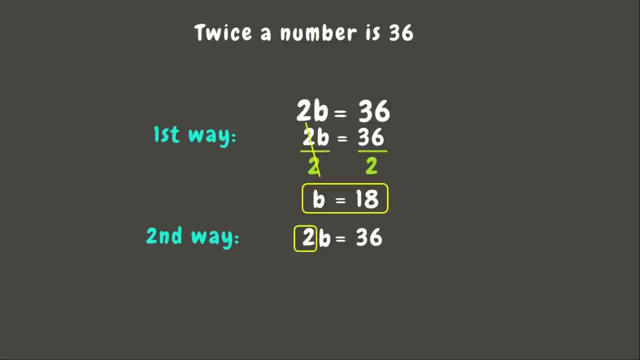 We are just simply going to move it on the other side of the equation By dividing the other side by the coefficient. There you go. So that gives us b equals 36 divided by 2, which is 18.. Great job. Now to check our answer. 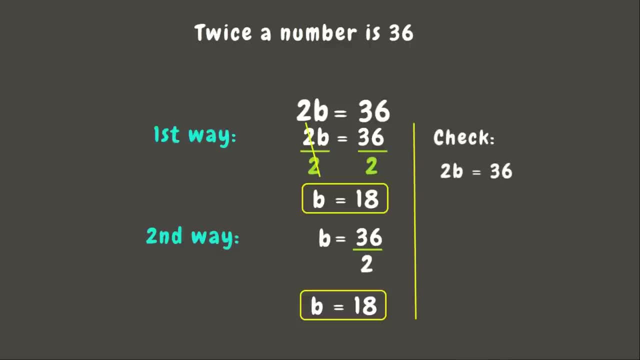 Let us substitute the value of the variable. Now our answer is correct. Now let's go and have another example This time. we have n divided by 8 is 11.. So let us translate this one first. We have n divided by 8.. 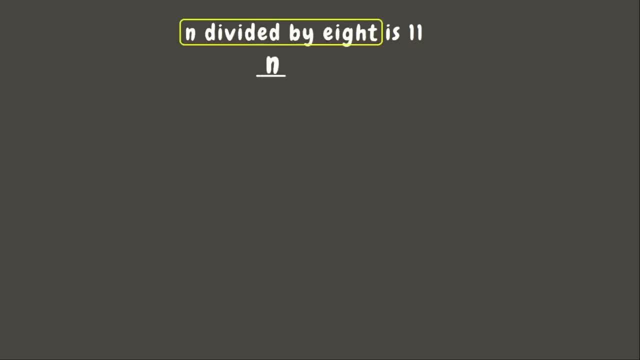 Which means n over or divided by 8 is equal 11.. Again, the first thing that we need to do is to separate or leave alone the variable on one side. So this means we need to get rid of our constant, which is 8.. 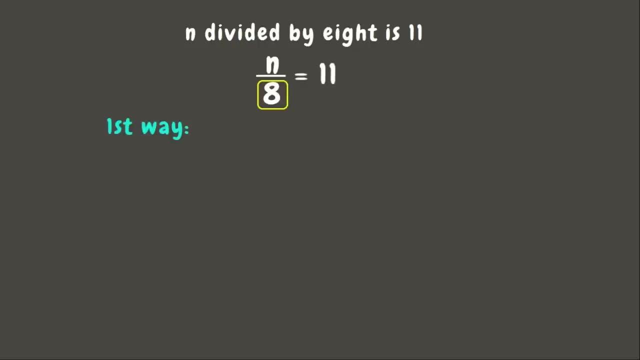 But how are we going to do that? So let's try our first way. We have n divided by 8 equals 11. To get rid of the constant 8. We are going to get its opposite operation, Since it is division. the opposite would be multiplication. 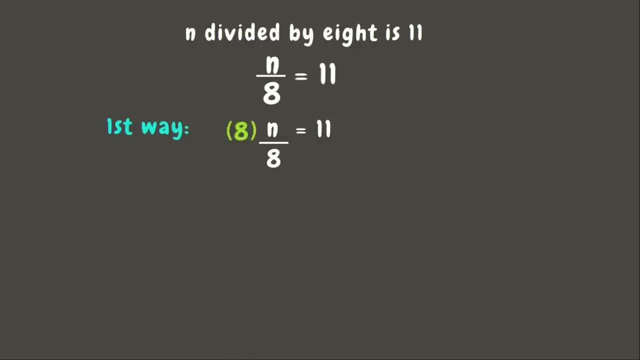 So we need to multiply 8 on both sides. There you go. Now let us solve. We have 8 divided by 8, which is 1.. So we can simply cancel this out. So that leaves us the variable n equals 11 times 8, which is very good: 88.. 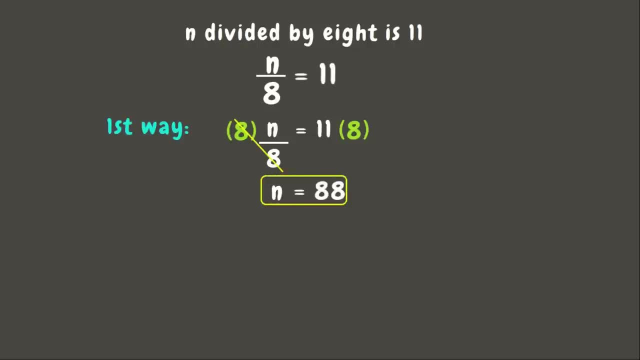 So that is the value of our variable. Now let's solve our second way. In our second way, we are going to get the opposite operation of our constant, which is 8.. And its opposite operation is multiplication, And the next thing that we are going to do is to move it on the other side of the equation. 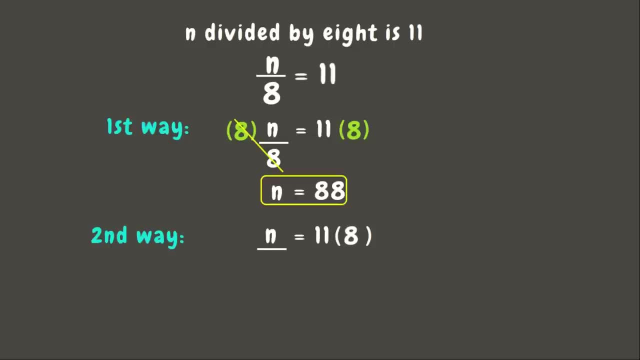 There you go. Now that is n equals 11 times 8, which is 88.. Good job. Now let us check our second way. Now let us check our answer. Now, our answer is correct. Now let's have another example. This time we have twice a number. 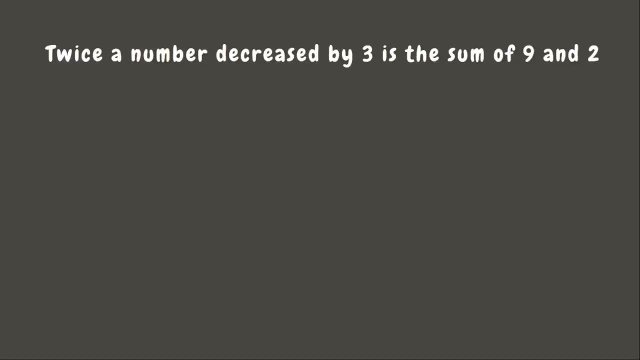 Decrease by 3, is the sum of 9 and 2.. Let us translate this one first into one equation. So we have first twice a number And that means 2 times a variable. So that would be 2 times x or 2x. 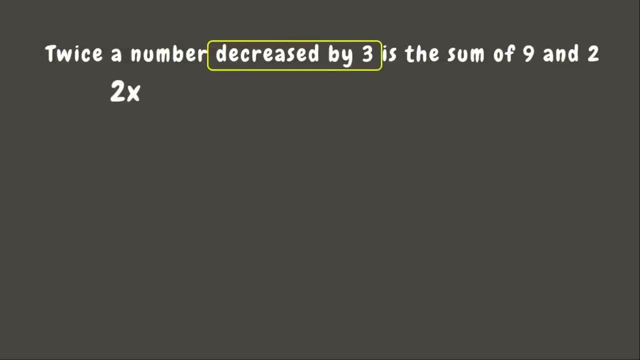 Next one: we have decrease by 3, which means subtraction, So that is minus 3.. And on the other side we have is the sum of 9 and 2, which is equals 9 plus 2.. As you can see, we have operations on both sides. 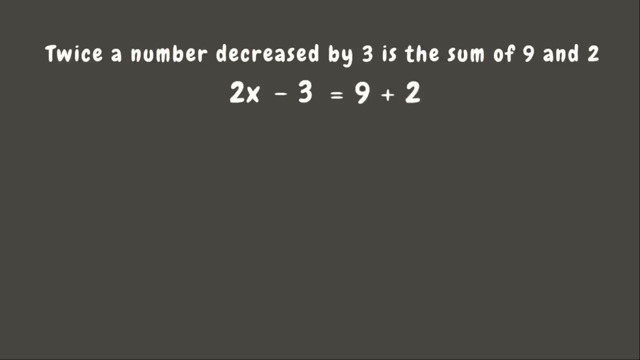 Before we can find the value of the variable, we need to simplify first anything that we can simplify on both sides. So here we can simplify 9 plus 2, which is 11. While on the other side that leaves us 2x minus 3.. 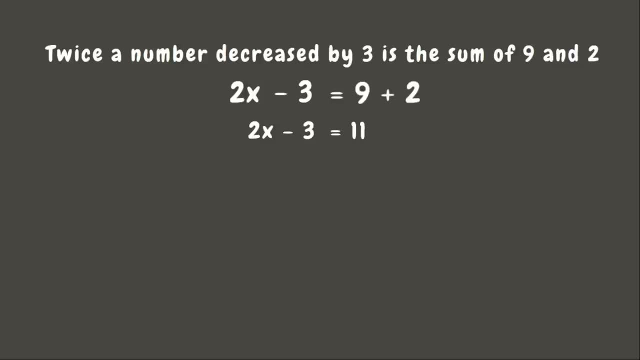 Now let us try to solve for the variable by getting rid of all the constants and the coefficient. Remember, the first thing that you need to get rid of is the addition or subtraction. So since we have here subtraction which is minus 3., Let's remove this one first by getting its opposite operation, which is plus 3.. 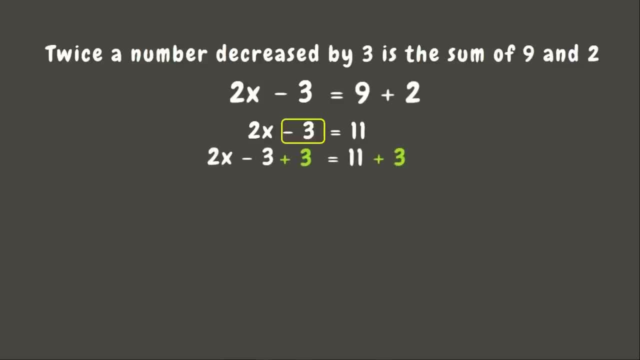 Now let's add 3 also on the other side, So that is 11 plus 3.. Now we have negative 3 plus 3, which is 0. So we can simply cancel this out And that leaves. 2x equals 11 plus 3, which is 14.. 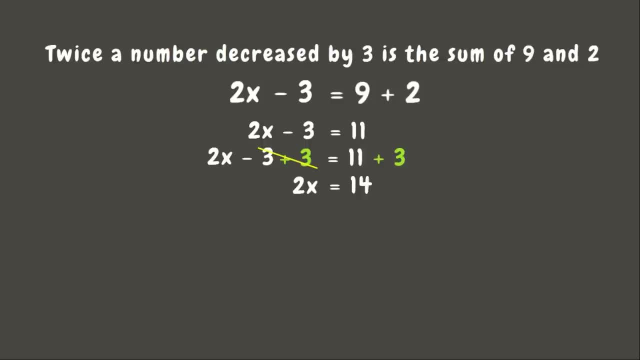 Now we only have one operation left, which is multiplication, and that is 2 times x. Now, to get rid of the coefficient 2, we are going to get its opposite operation, which is division. So let us divide 2 on both sides. There you go. 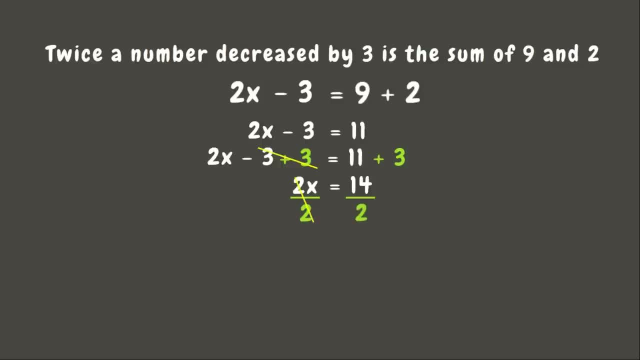 So we can cancel out 2 divided by 2, since it is equal to 1.. And that leaves us the variable. x equals 14 divided by 2, which is 7.. Great job, Now the value of our variable is 7.. 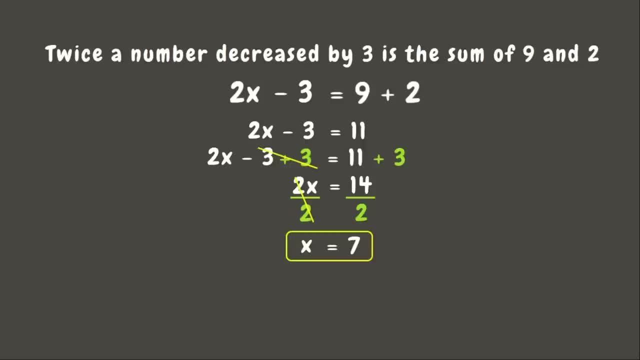 Now let us check if our answer is correct. Great job. Now let's have another example. This time we have 2 more than the quotient of n, and 4 is 8.. Now let's translate this again into one equation. So we have 2 more than, which means addition, and that is plus 2.. 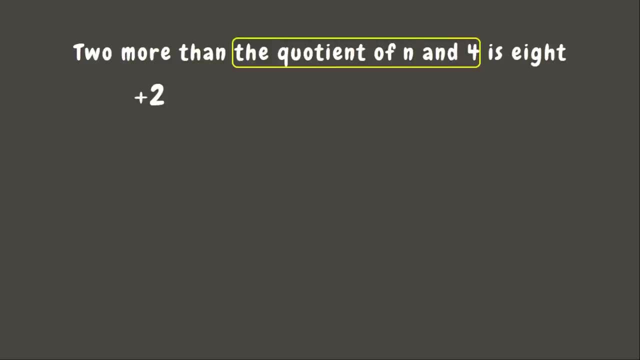 And next we have the quotient of n and 4, which means division, So that is n divided by 4.. And lastly, we have is 8, which means equals 8.. Again, the first thing that we need to get rid of, to leave the variable alone on one side, is addition or subtraction. 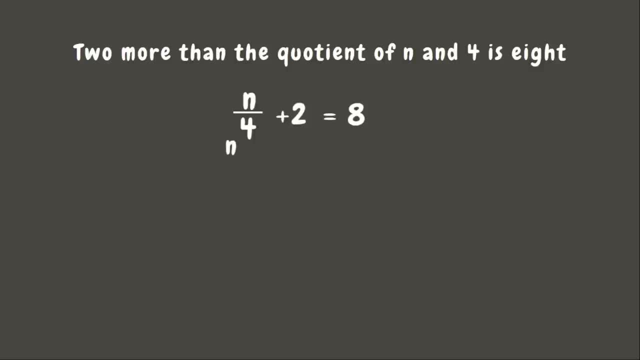 Since here we have addition, which is plus 2.. And its opposite operation is subtraction, which is minus 2.. We are also going to do that on the other side. Now let us solve. So we have positive 2 minus 2.. So we have: 2 minus 2 equals 0.. 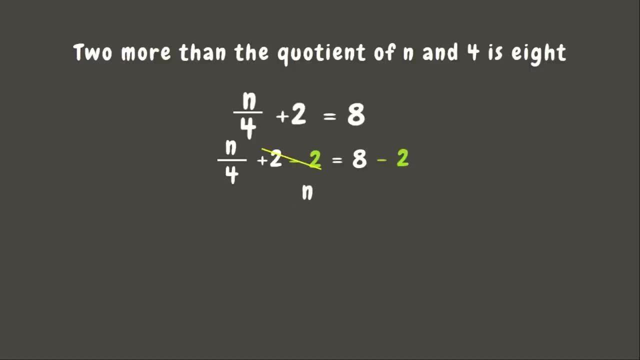 So let's cancel this out. and that leaves us n divided by 4.. Equals 8 minus 2, which is 6.. Now we are down to our last operation, which is division. To cancel out the constant 4, we are going to get its opposite operation, which is multiplication. 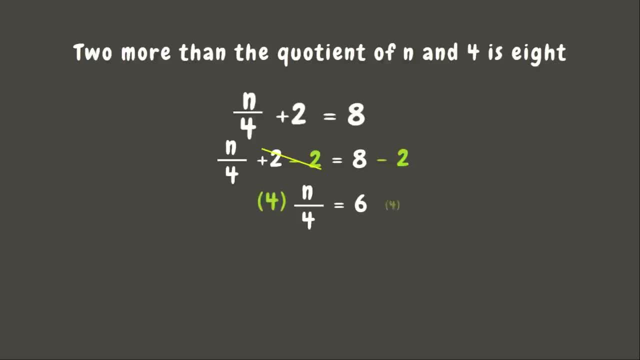 So we need to multiply 4 on both sides. Now let us cancel out 4 divided by 4, since its equal 1.. And that leaves us the variable n Equals 6 times 4, which is 24.. Great job. Now let us try to check our answer. 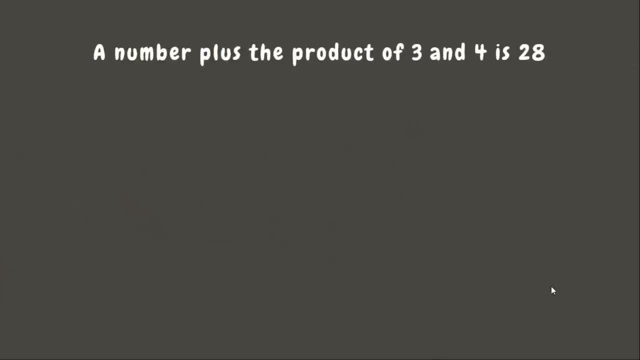 There you go. Now we are down on our last example. This time we have a number plus. the product of 3 and 4 is 28.. So let's translate this one, Let's translate this one first into one equation. So first we have a number plus. 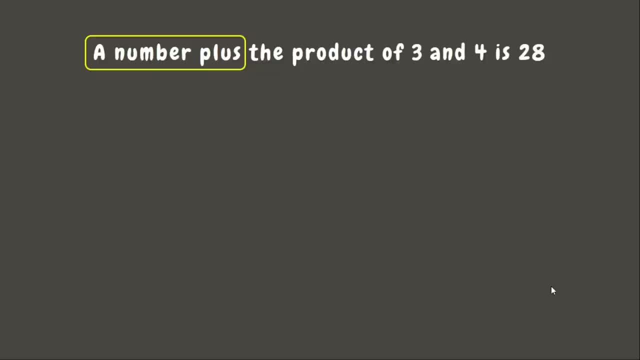 So a number means a known. So let us represent this by a variable. Let us say h, So that is h plus, And next we have the product of 3 and 4, which means multiplication, So that would be 3 times 4.. 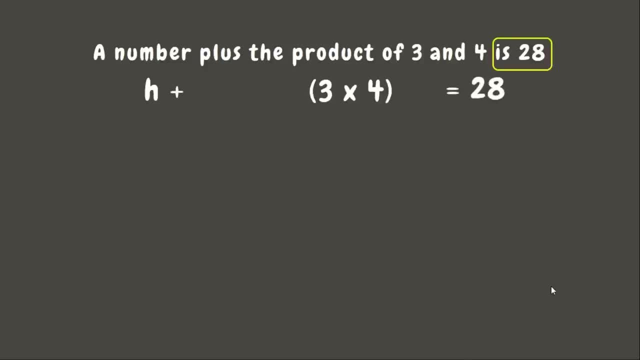 And lastly we have is 28, which means equals 28.. Now our equation is: h plus Plus, the product of 3 and 4 equals 28.. Now, first, again, we need to simplify anything that we can simplify on both sides, Since we can already simplify 3 times 4.. 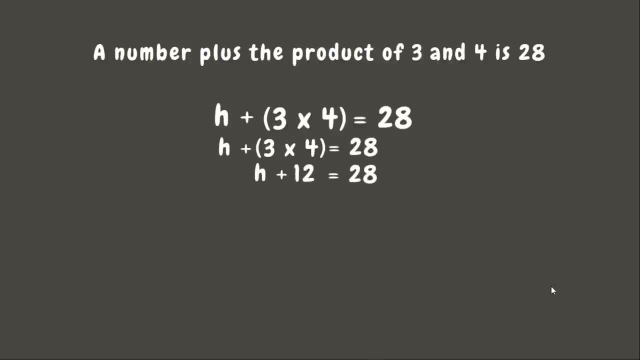 We all know that that is 12.. So now we have: h plus 12 equals 28.. Let's get rid of our constant by getting its opposite operation. So, since it is addition or plus 12, we need to subtract 12 on both sides. 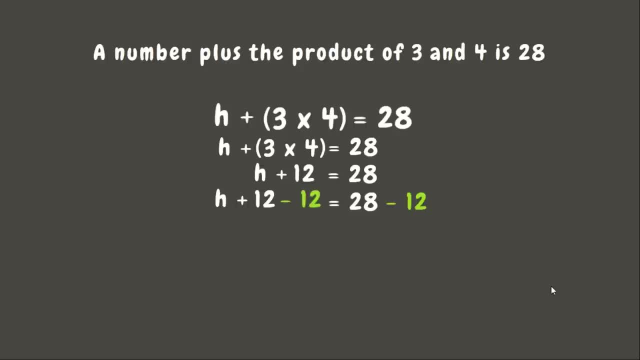 There you go. Now let us simplify. So we have 12 minus 12, which is 0. So let us cancel this out And that leaves us the variable. h Equals 28 minus 12, which is 16.. And that is the value of our variable. 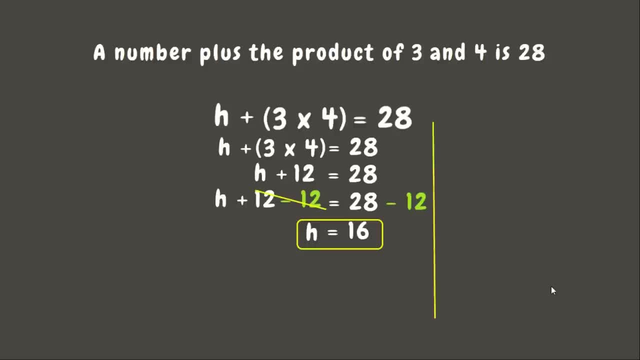 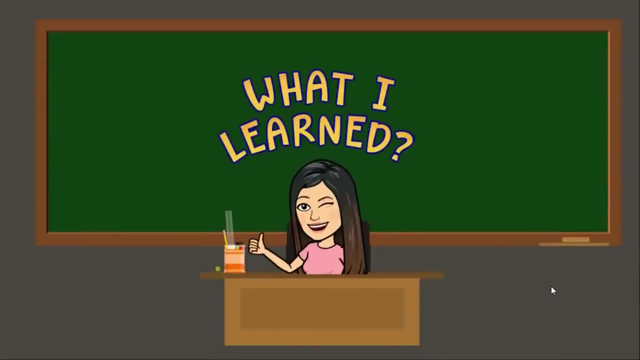 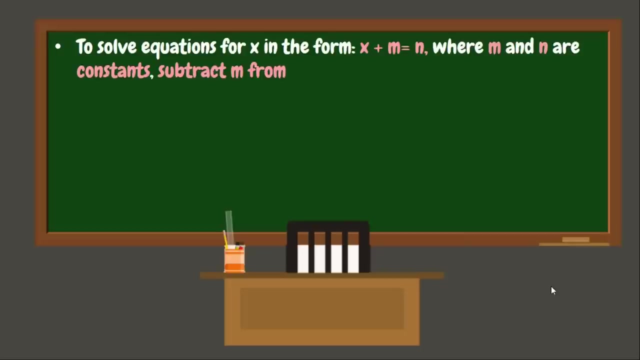 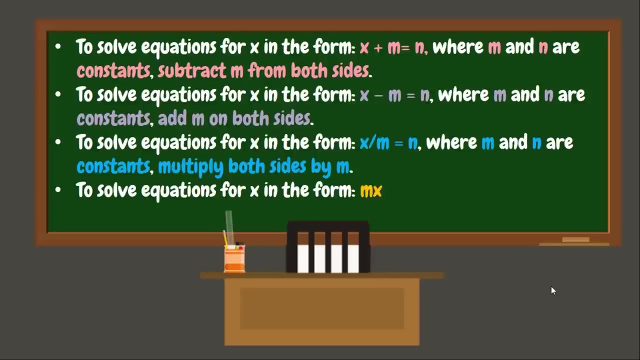 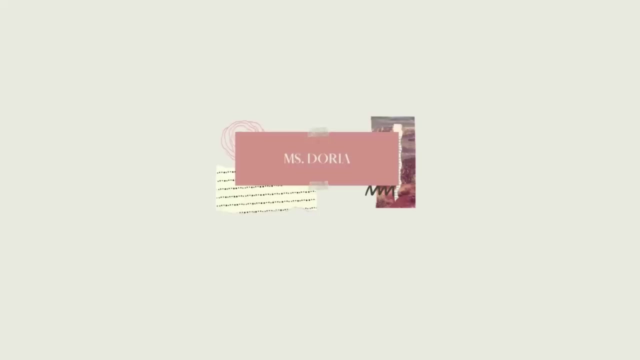 Now let us check if our answer is correct. Great job, Wonderful. Now here are the things that you learned today. Thank you very much for watching.